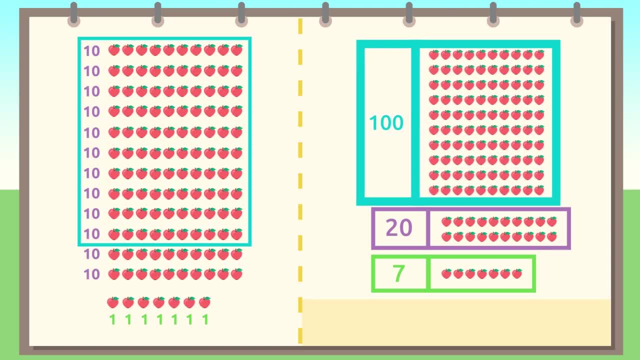 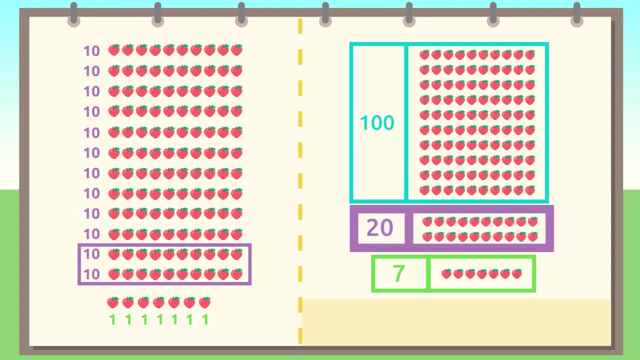 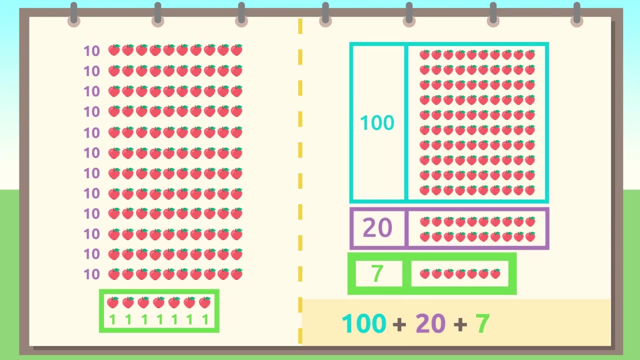 10 groups of 10 apples each gives me 100 apples. Then I have 2 groups of 10 apples and 7 single apples left over, Meaning 100 plus 20 plus 7 equals 127 apples. Amazing, I can group the apples by 10 or group them further by 100 to quickly count large quantities. 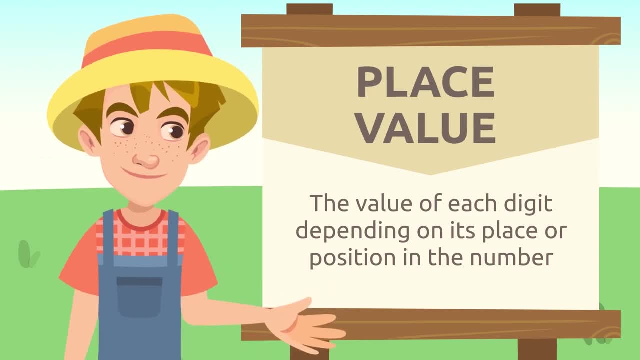 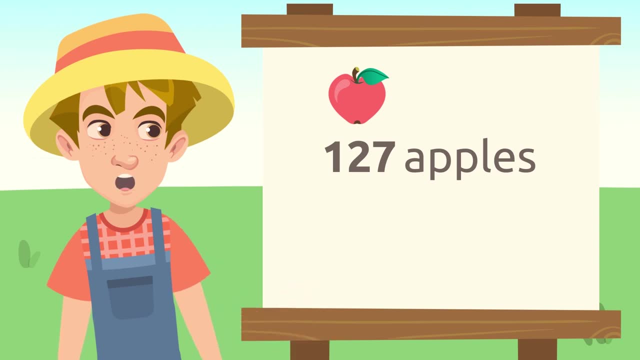 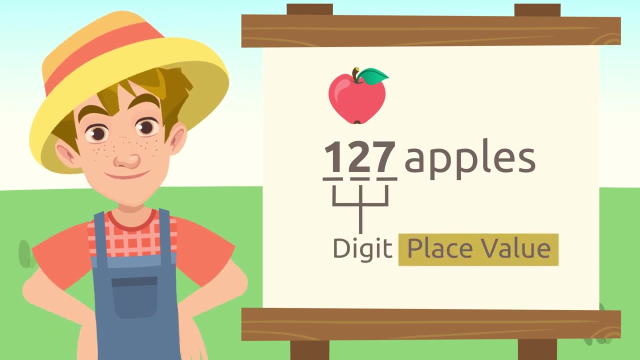 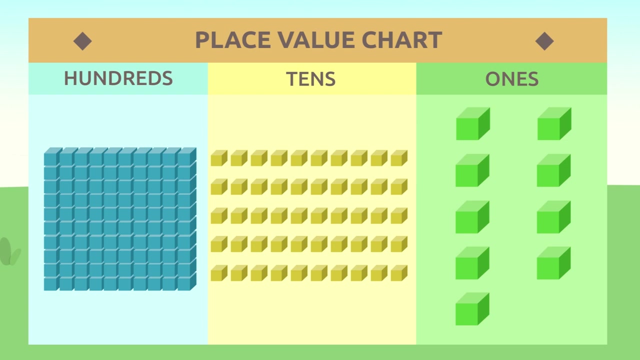 Did you know that each digit in a number has a meaning? This is called place value. We counted 127 apples. Each digit- 1,, 2, and 7- has a place value. Let's look. We use a place value chart to show the place value of each digit. 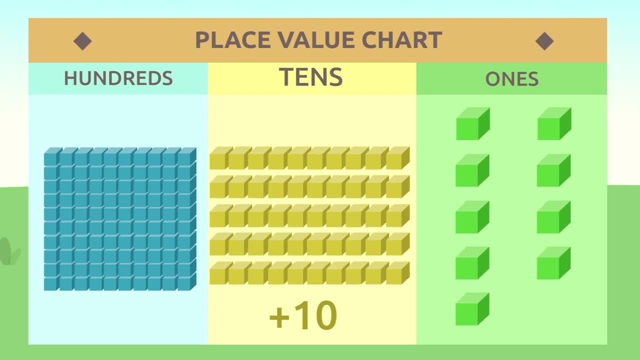 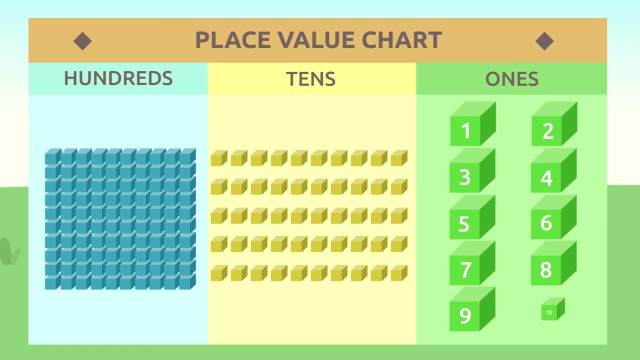 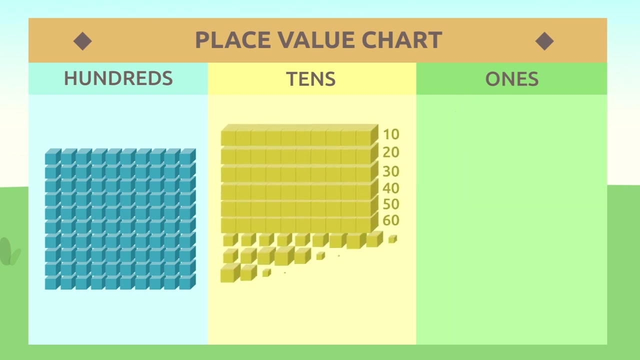 This is 1's place, 10's place And 100's place. We count till 9 under 1's place. When we get to 10, we move to the 10's place. We continue counting till 99.. 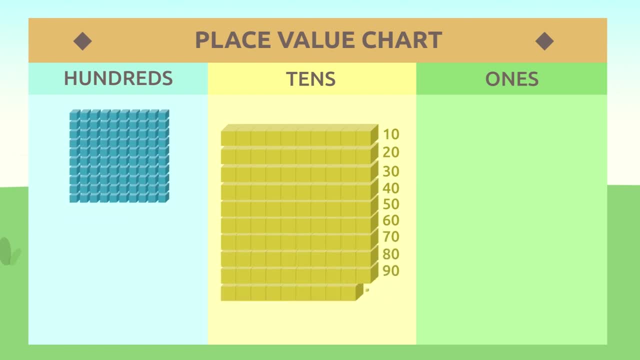 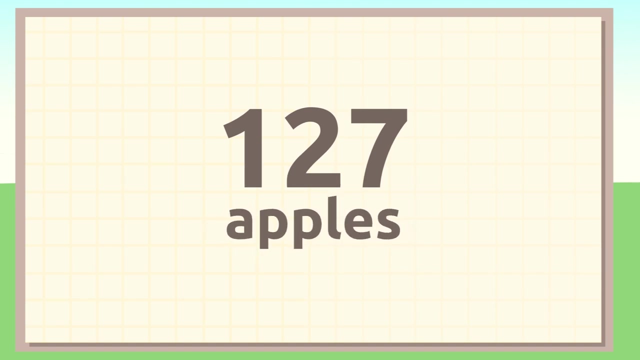 When we get to 100, we move again to the 100's place. As you can see, the place value increases as we go from 1's to 100's. Since we counted 127 apples earlier, we can place 7 single apples under 1's value. 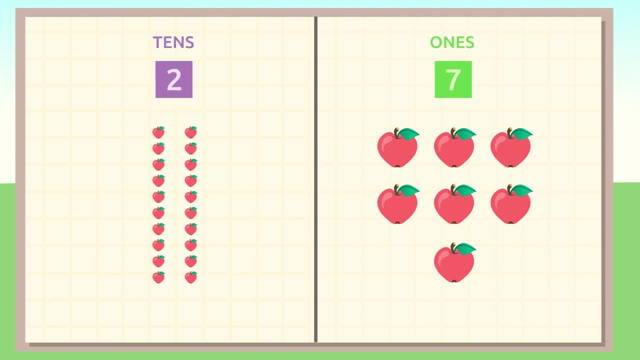 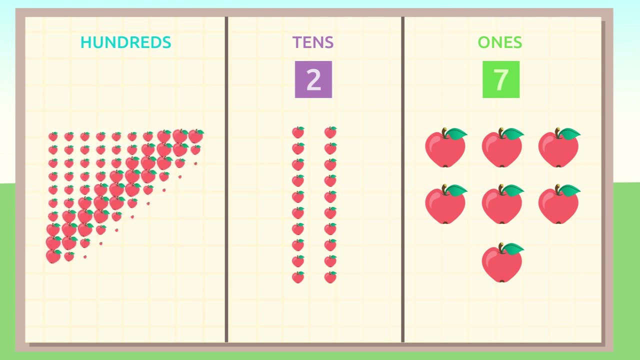 We had 2 groups of 10 apples, so we can place the 2 groups under the 10's value. Finally, we had 1 group of 100 apples which we made with the 10 groups of 10 apples. We can place the 1 group under the 100's value. 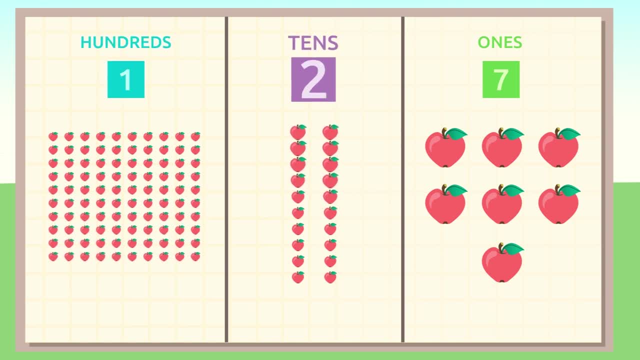 1 is in the 100's place, 2 is in the 10's place And 7 in the 1's place. 100 apples plus 20 apples plus 7 apples gives us 127 apples. Cool huh. 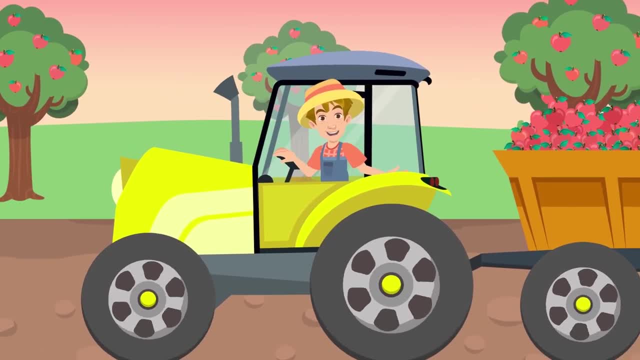 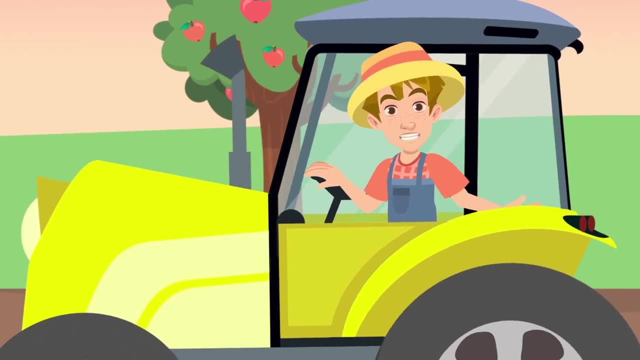 I've finished counting all these apples. Grouping the apples 10 and 100 was a great idea. So was using the place value. Grouping the apples 10 and 100 is a great idea. place value chart to put the digits in the correct place values: ones, tens and hundreds. 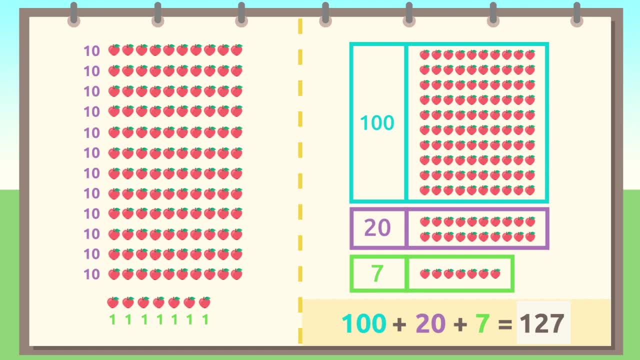 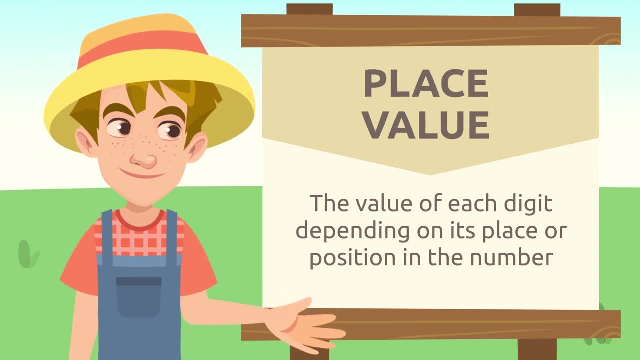 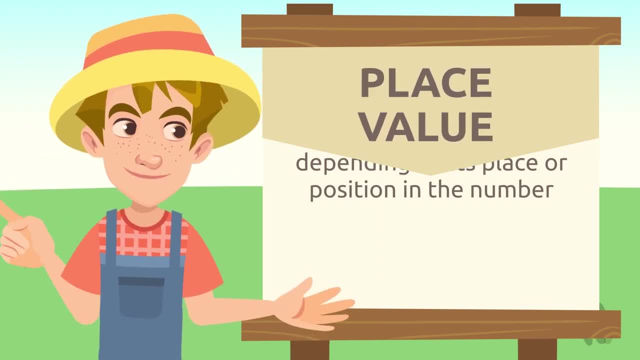 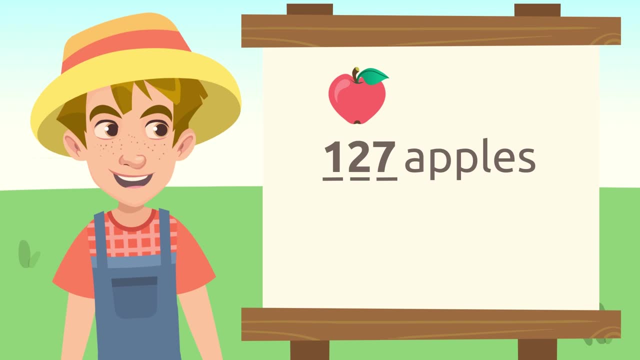 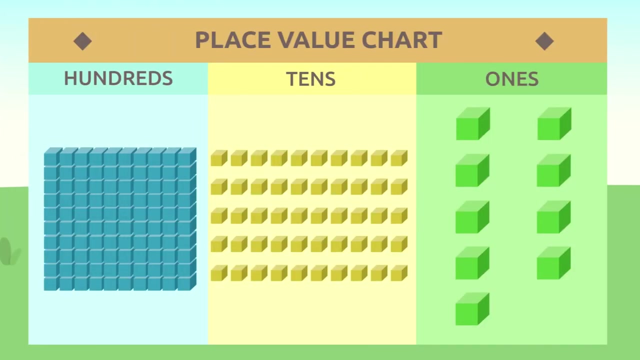 This is called place value. We counted 127 apples. Each digit 1,, 2, and 7 has a place value. Each digit 1,, 2, and 7 has a place value. Let's look. We use a place value chart to show the place value of each digit. 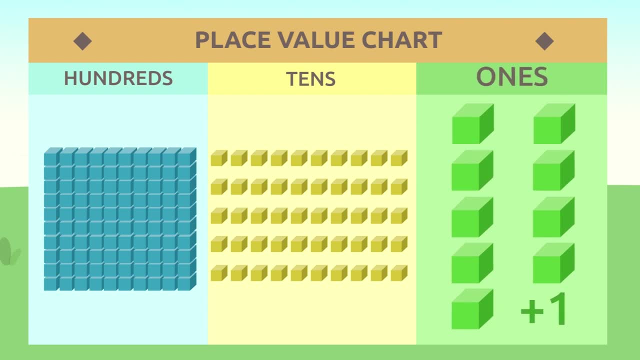 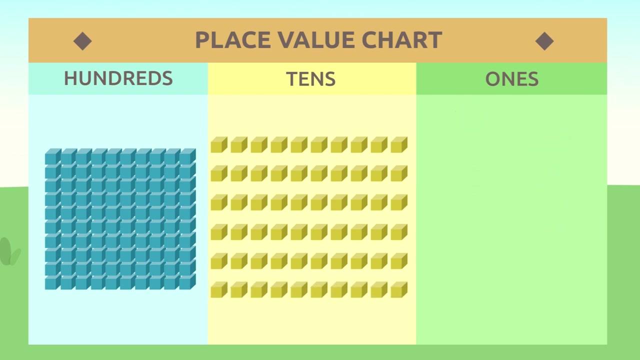 We use a place value chart to show the place value of each digit. This is 1's place. This is 1's place, tens place and hundreds place. We count till nine under ones place. When we get to ten, we move to the tens place. We continue counting till 99.. When we get to. 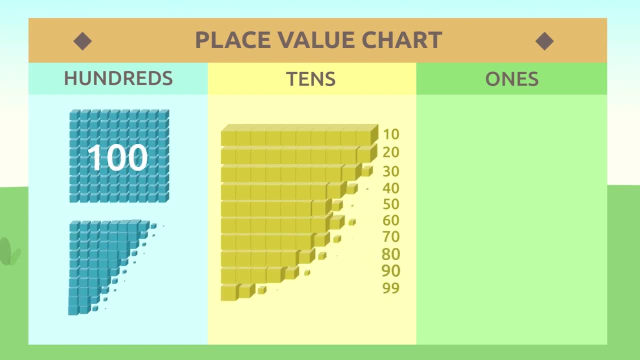 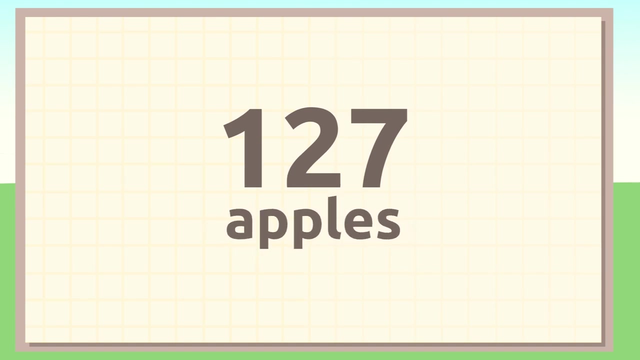 a hundred, we move again to the hundreds place. As you can see, the place value increases as we go from one to hundreds. Since we counted 127 apples earlier, we can place seven single apples under ones value. We had two groups of 10 apples, so we can place the two groups. 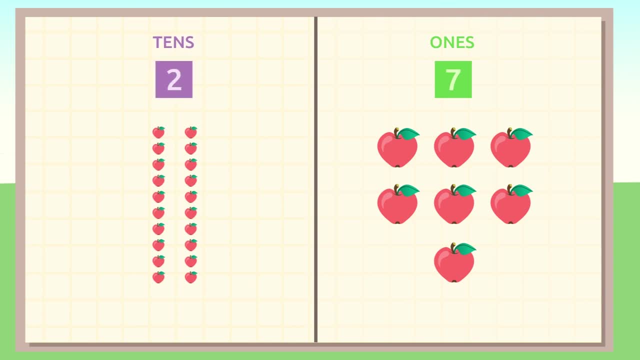 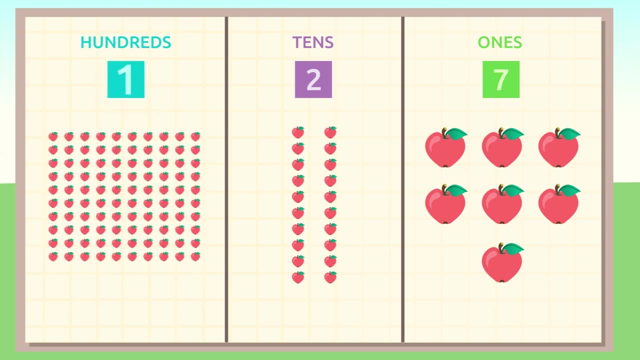 under the tens value. Finally, we had one group of 100 apples which we made with the ten group of 10 apples. We can place the 1 group under the hundreds value. 1 is in the hundreds place, 2 is in the tens place and 7 in the ones place. 100 apples plus. 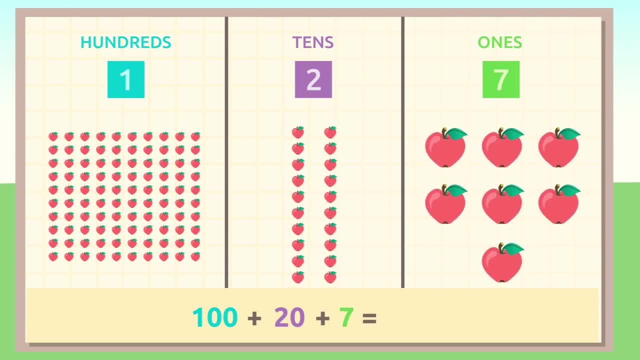 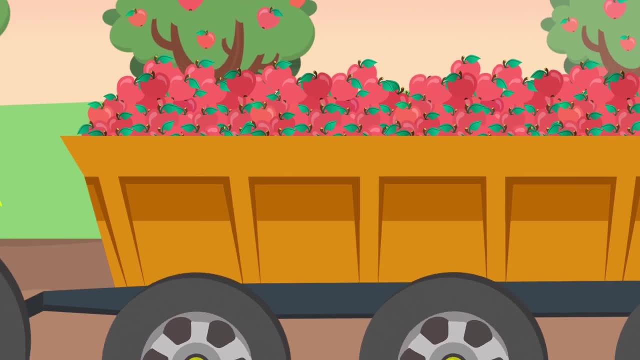 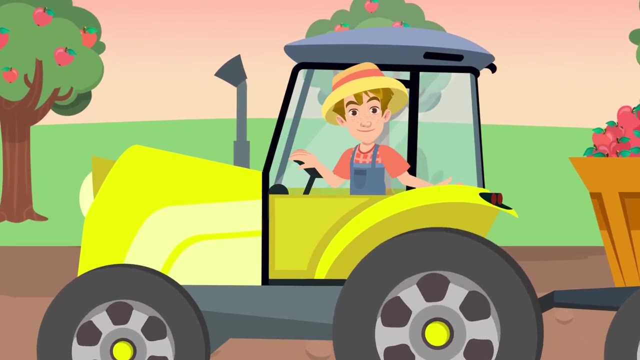 20 apples plus 7 apples gives us 127 apples. Cool huh. I finished counting all these apples. Grouping the apples by 10 and by 100 was a great idea, So was using the place value chart to put the digits in the 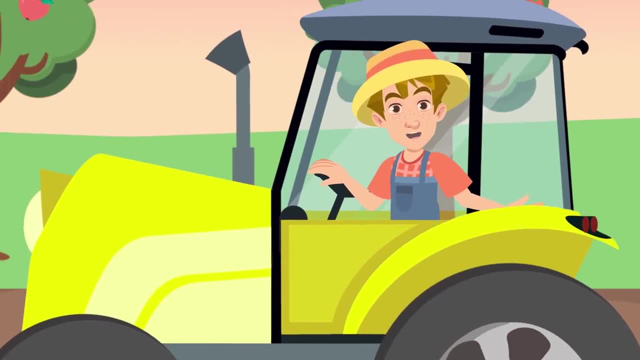 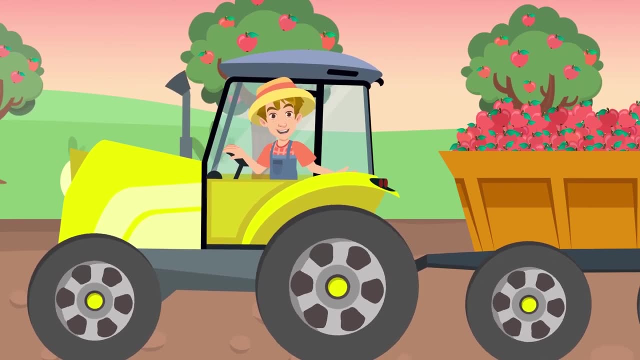 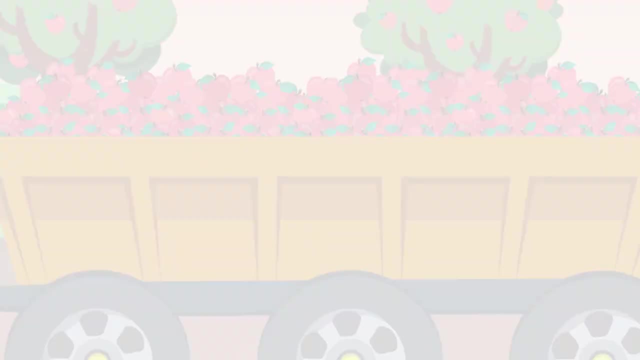 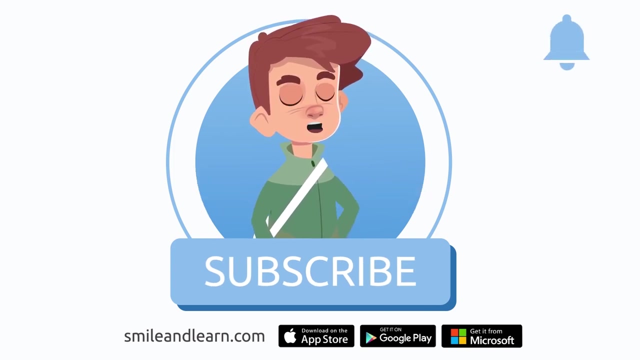 correct place values: Ones, tens and hundreds. This made counting all the apples way easier. Thank you for helping me today. Time for some apple pies. See you later. We've learned so much in just one video. Did you know there are many more videos? 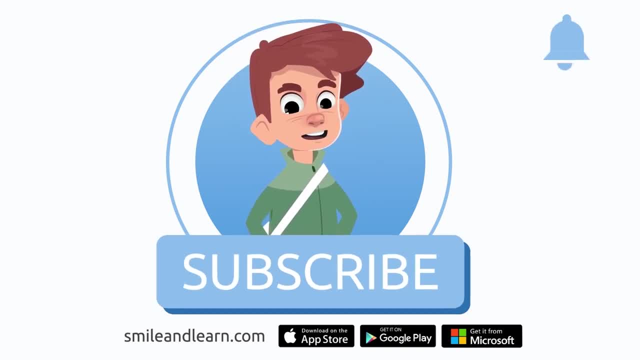 Imagine how much you could learn. Subscribe to the Smile and Learn educational channel to learn and have fun at the same time. 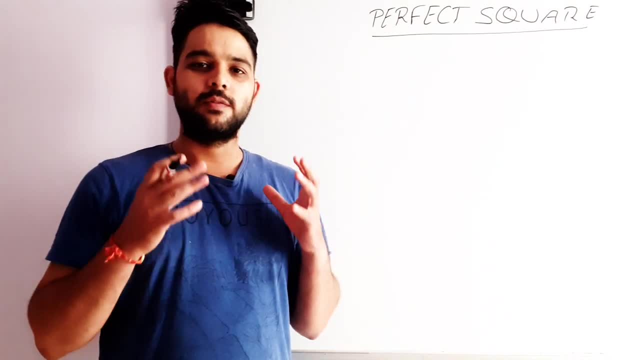 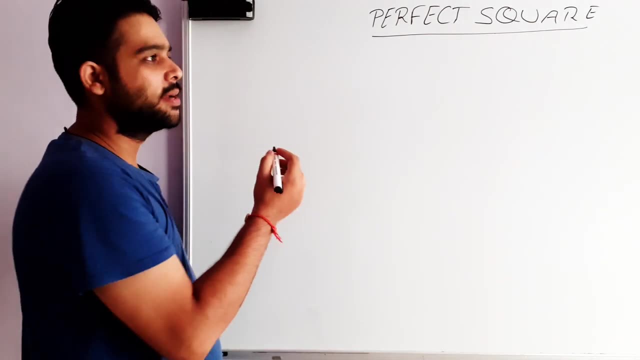 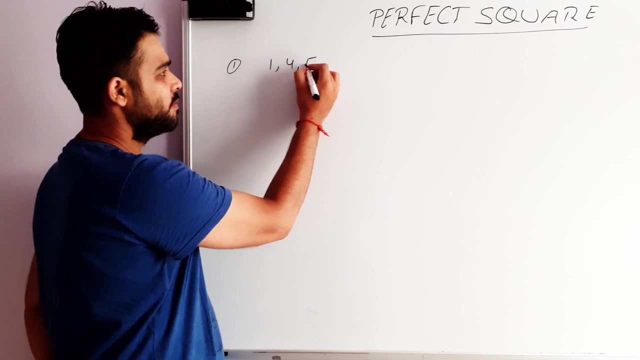 Hello everyone. So in this video I am going to tell you how you can find whether a number is a perfect square or not. So we will start with the basics. A perfect square always ends in the following numbers. This means 1,, 4,, 5,, 6,, 9 and 0.. So a perfect square will always. 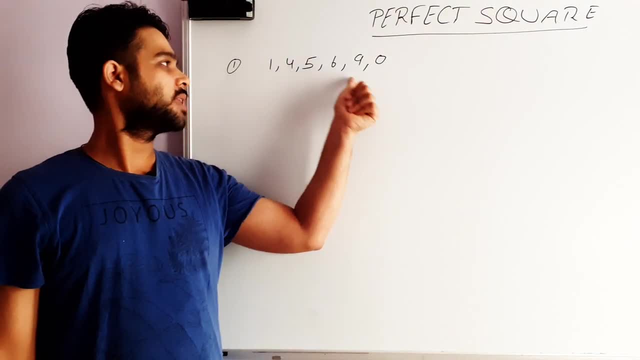 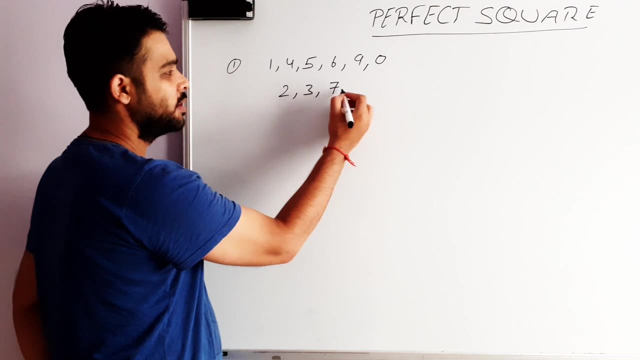 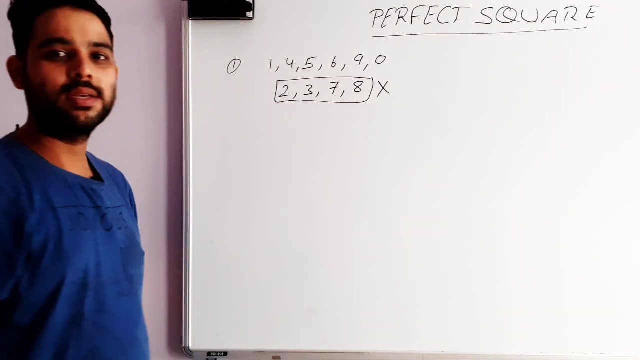 end in either 1,, 4,, 5,, 6,, 9 or 0. This means if you have the last digit as 2,, 3,, 7 or 8, the number will not be a perfect square if the last digit is 2,, 3,, 7 or 8.. Second important: 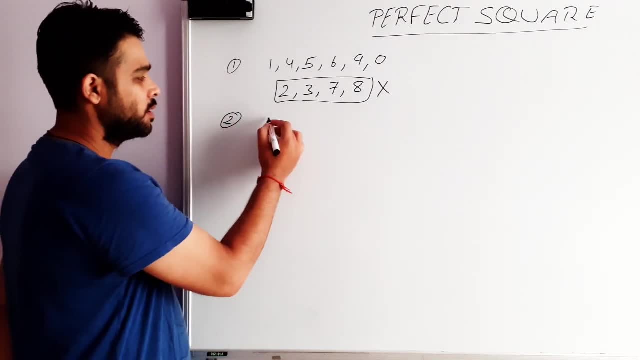 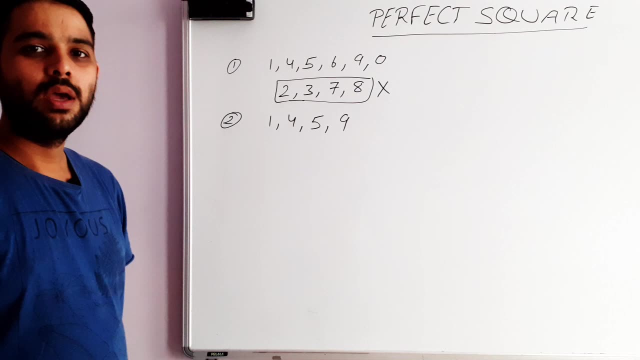 thing: if you have the last digit as 1,, 4,, 5,, 6,, 9 or 0,, then the number will not be a perfect square. If the last digit of an answer is 1,, 4,, 5 or 9,, then the second last. 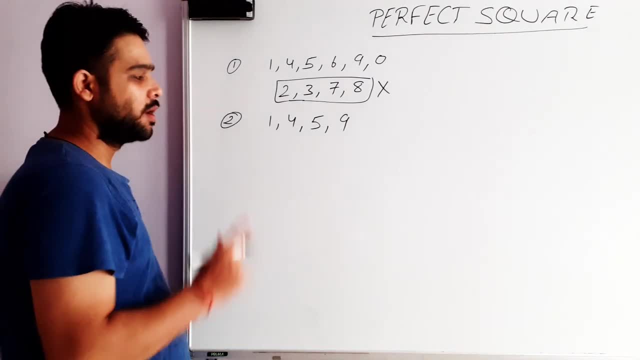 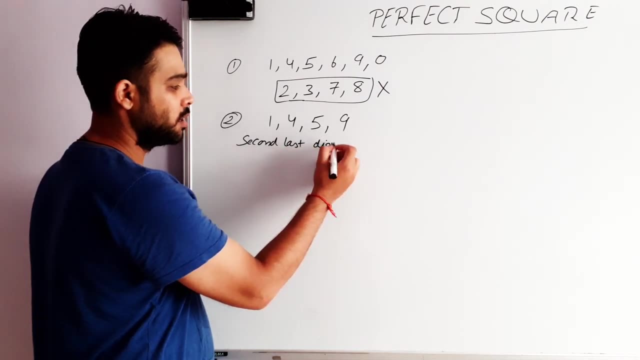 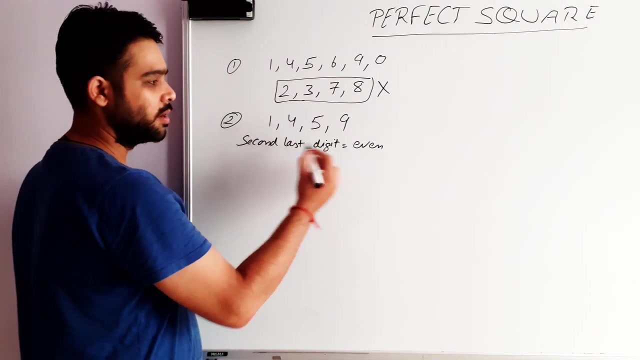 digit will always be an even number for a perfect square, For example. second last digit is: even If the last digit is 1,, 4,, 5,, 9.. I will give you an example. You take any number, just say 1,, 4,, 5,, 9.. If the last digit is 1,, 4,, 5,, 9, then the number will not be a.